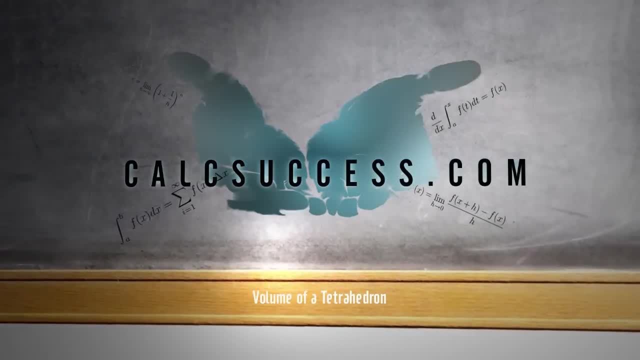 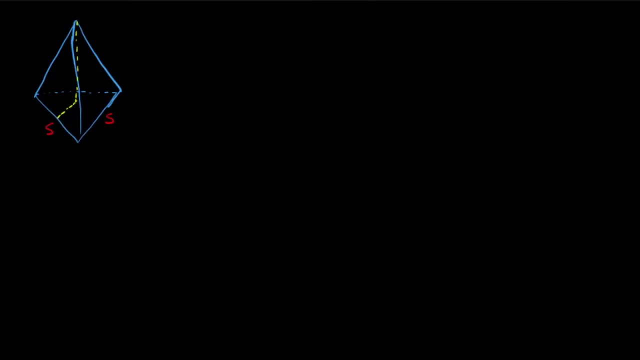 Okay, so our task is to find the volume, derive the formula for the volume of this tetrahedron, And so we're assuming that the face, each one of these faces, is an equilateral triangle of length s. So let's take a look at a cross section here And what I'm going to do to 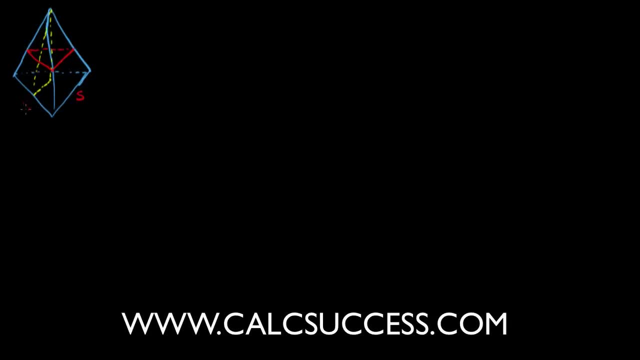 kind of help me come up with a formula for the area of the cross section, which is essentially what I want to do. I'm going to call these sides. I'm just going to assume that these aren't the same. So I know it's an equilateral triangle, but I'm going to call them just. 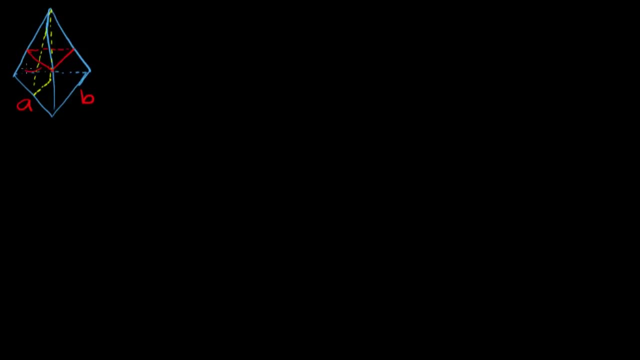 a and b. So for now and then, I'm going to call this one alpha and beta to correspond with these a and b, And I'm going to say that the height of the tetrahedron is h and then the height from the bottom to where the cross section is located is going to be y. 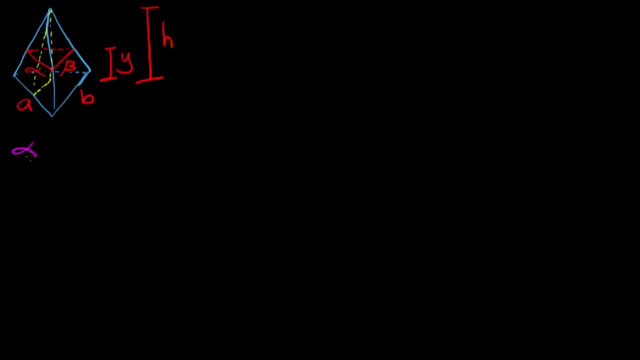 And so triangles. I know that alpha over a is equal to beta over B. so then alpha is equal to a times beta over B. now we also, again using similar triangles, we can see that H over B. so the total height over this side is going to be proportional to. 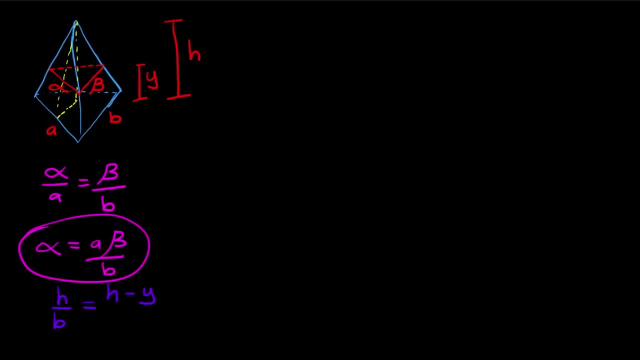 H minus Y, so that's the height from the tip to our triangle, H minus Y over beta. and so then from this we can see that beta is going to equal to B times H minus Y over H, and so then alpha is equal to a times beta over B, so this is a times B, H minus Y over H. so 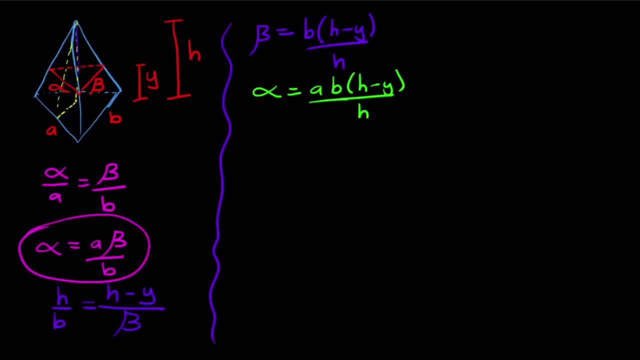 this part right here is beta, and then over the B. that's right there from alpha. so then notice that the B's cancel, and so then alpha is equal to a times H minus Y over H. okay, so now let's take a look at our cross-section again. so let's. 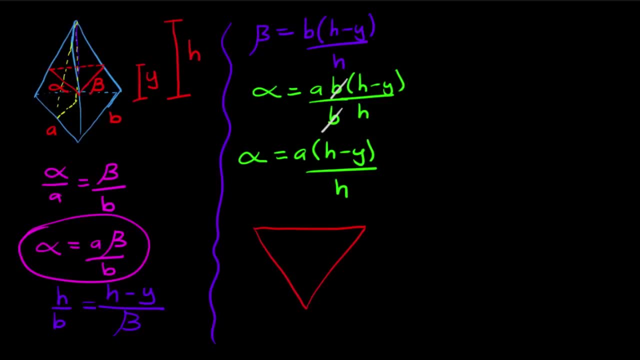 go back to our cross-section again. so let's go back to these. this is an equilateral triangle, so these: this is an equilateral triangle, so these: this is an equilateral triangle, so this guy's site is alpha, and then this guy's site is alpha, and then 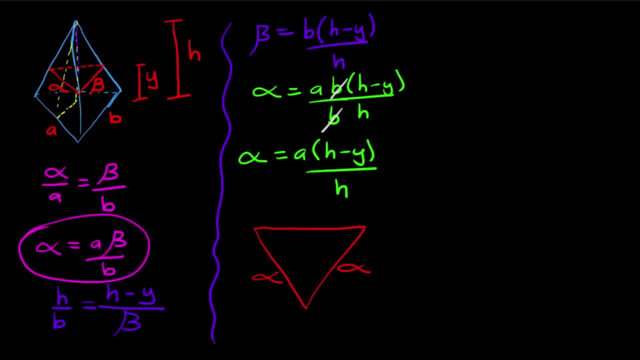 this guy's site is alpha. and then, remember, here we labeled it beta. but remember, here we labeled it beta. but remember, here we labeled it beta, but it's really an equilateral triangle and it's really an equilateral triangle and it's really an equilateral triangle, and so that's alpha as well. so, since what I 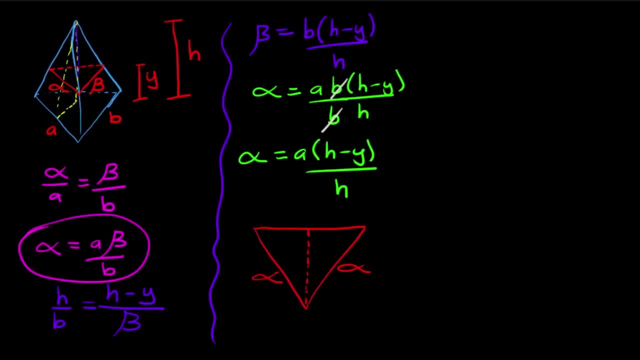 so that's alpha as well. so, since what I so, that's alpha as well. so, since what I want is to do is to find the area of want is to do is to find the area of want is to do is to find the area of this triangle, then what I need to do is 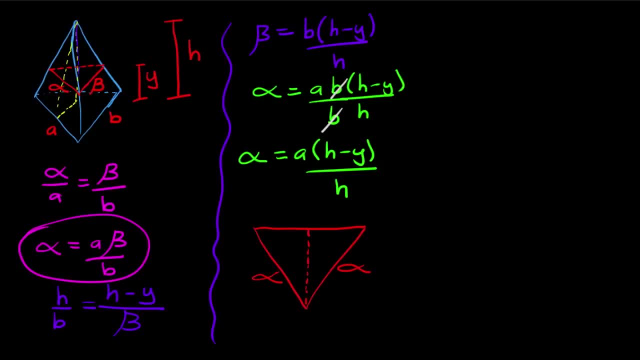 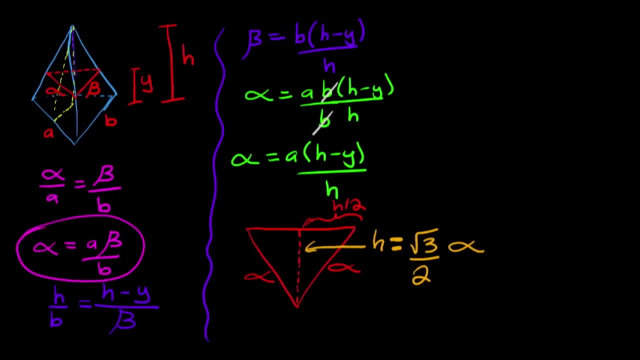 this triangle, then what I need to do is find the, the height. so this side right here is h over 2, and so then, using the Pythagorean theorem, we can easily find that the height is equal to square root of 3 over 2 times alpha. okay, and so then the area of the cross-section is equal. 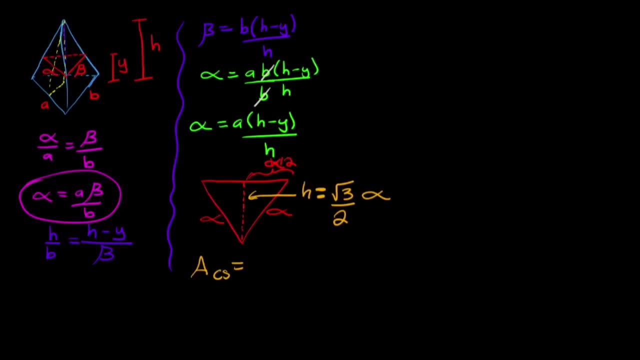 to. I'm sorry, this is alpha over 2, so the area of the cross-section- sorry about that- is 1 half the base, which is alpha, over here to here, times the height, which is root 3 over 2 alpha, and so then the area of the cross-section is 1 half 1. fourth root 3. 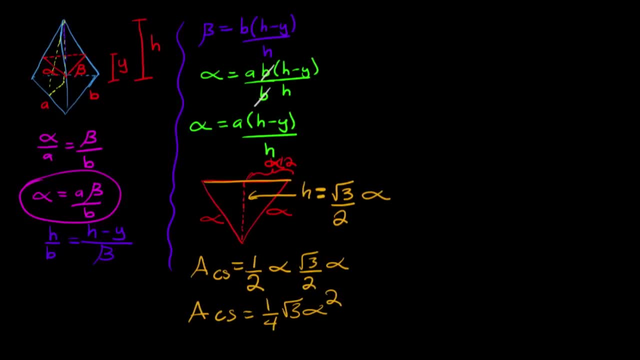 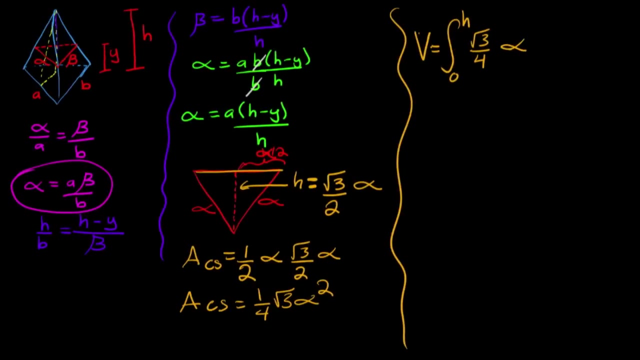 alpha squared. okay, so then the volume is simply equal to the integral from bottom to the top. so 0 to H of the square root of 3 over 4 alpha squared. but of course we don't want to use alpha because that's not our variable. variable is we're integrating. 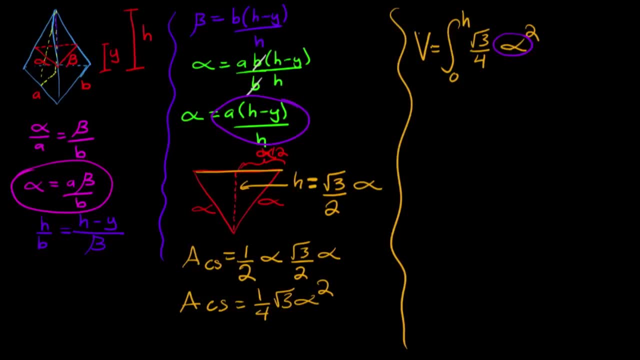 with respect to Y. so we're going to plug in that stuff right here in for alpha, and this is going to be with respect to Y, and we're going to plug in that stuff right here in for alpha, and so then what I have, I'm gonna put the constants on the outside square root of 3 over 4 and 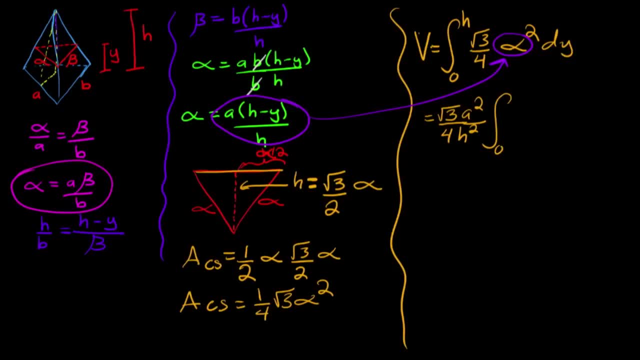 then I have a squared over h, squared because all this stuff is squared, then the integral from 0 to 18, h minus y, squared dy, and so this is equal to square square root of 3, a squared over four, and then minus 3. this is going to be a squared over 4, a squared divided by d times. if we subtract every other squared and then it's going to go up because all this stuff is squared, then 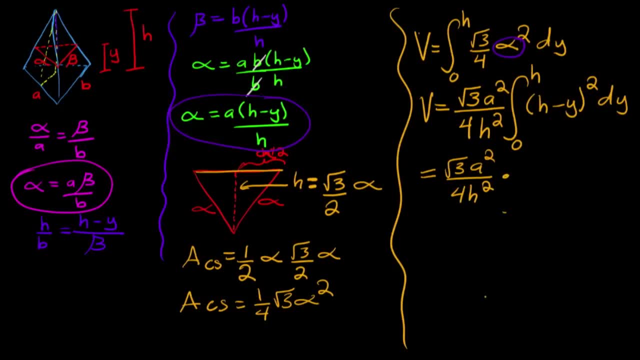 4H squared times. if you do this integral, you're going to get H cubed over 3.. And so with all this put together, you get the square root of 3 over 12 A squared times H, And that's the formula for the volume of that tetrahedron.